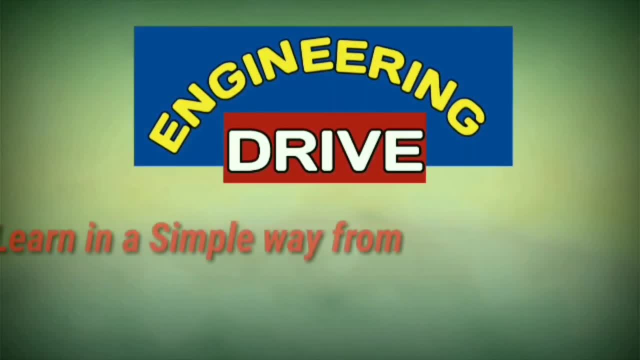 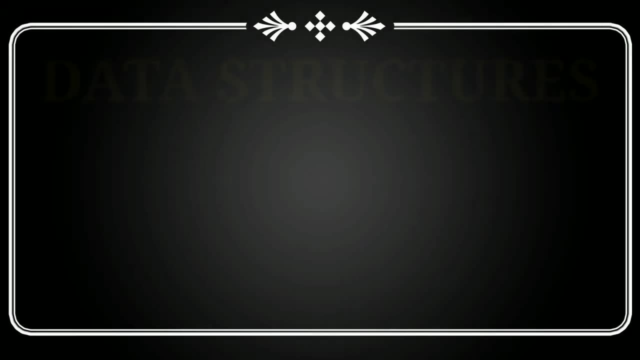 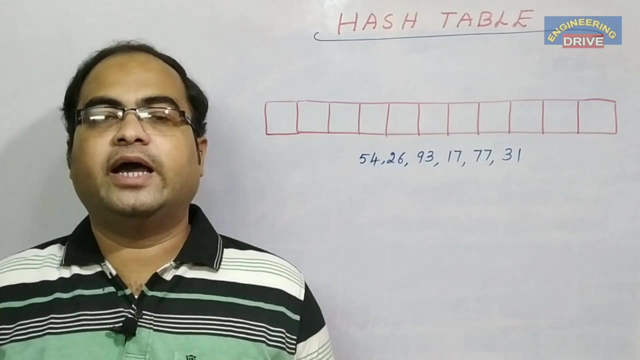 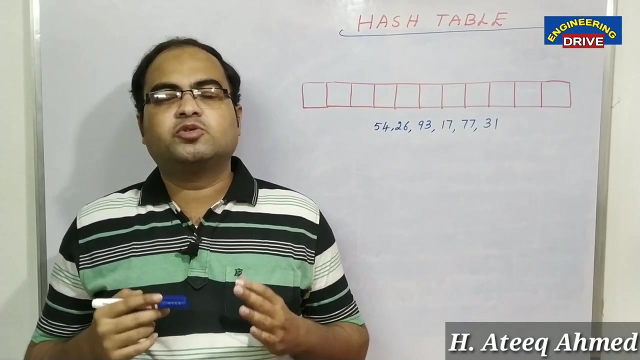 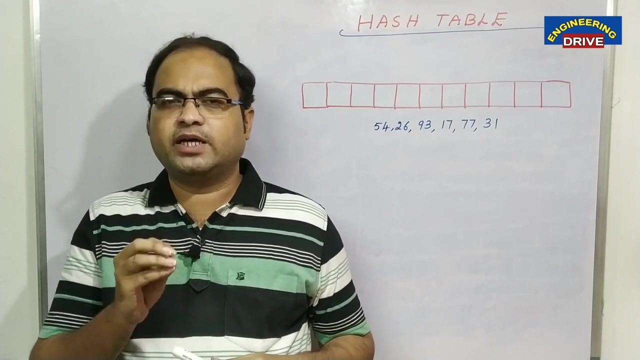 Hi, everybody, hope you are all fine. This is Atiq Ahmed. I welcome all of you to my YouTube channel, Engineering Drive. Today I am going to discuss about hash table. Hash table in data structures is one of those topics where most of the students they will face lot of difficulty in order to understand this much. 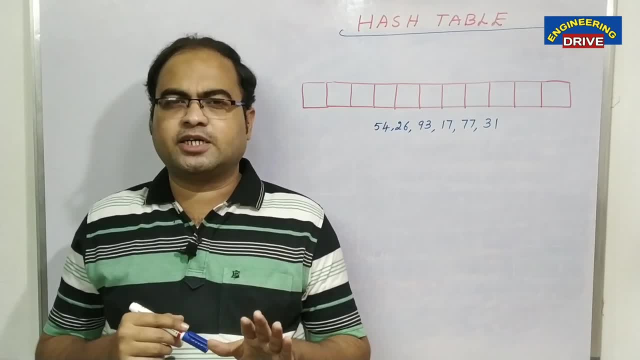 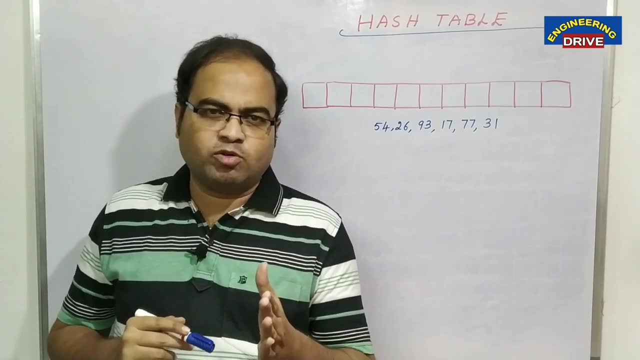 Ok, I don't know why, but I believe in data structures. one of the easiest and one of the interesting topic is hash table. Ok, now, if you are thinking now, if you are watching my video and if you are thinking that, sir, hash table is very difficult topic, sir, 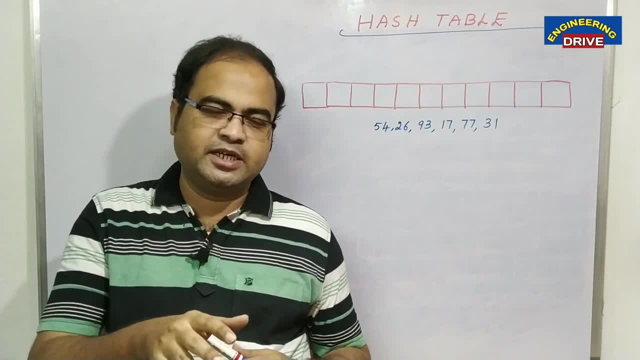 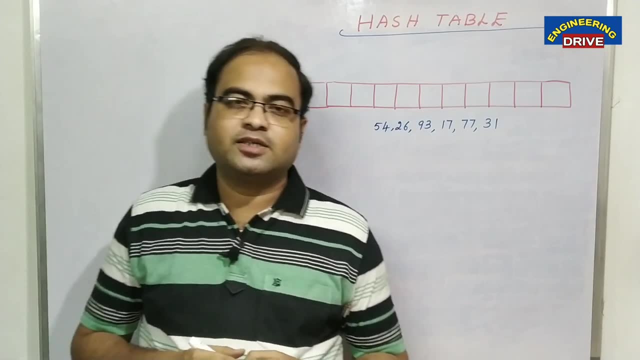 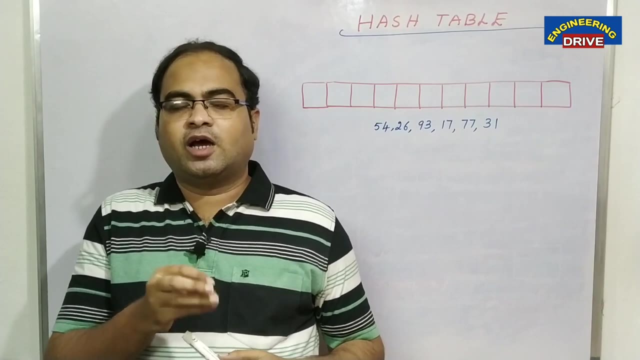 Then just tell me after 10 or 12 minutes whether it is easy or whether it is difficult one. Ok, surely put that in my comment section. Ok, now, my dear students, what is a hash table, why our computer makes use of hash table and how the data items can be stored in our hash table. 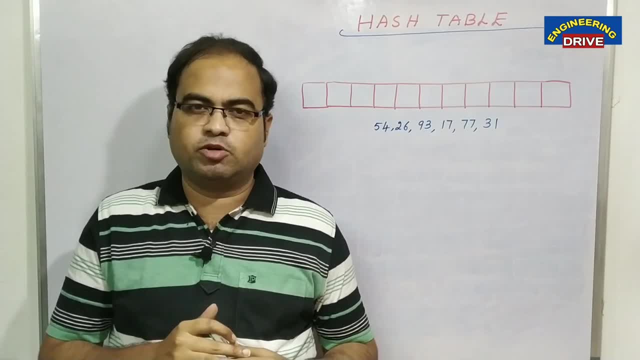 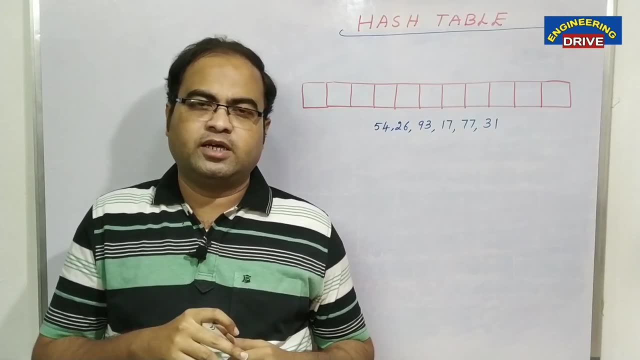 Ok, each and everything I am going to specify in my today's video. My dear students, hash table is also one type of data structures where the data is stored, Ok, and the data will be retrieved. Now, how the data will be stored in hash table that I am going to speak out now. 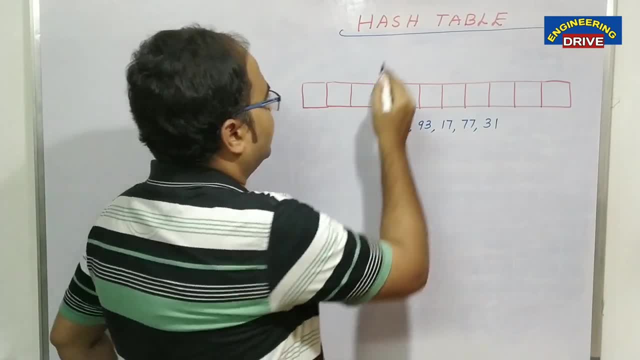 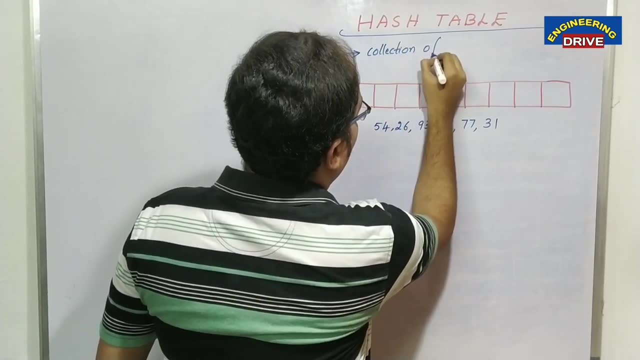 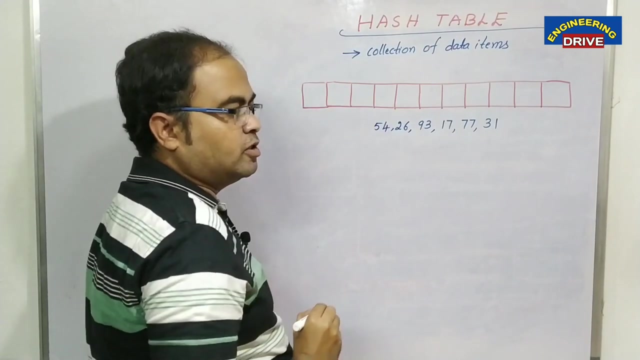 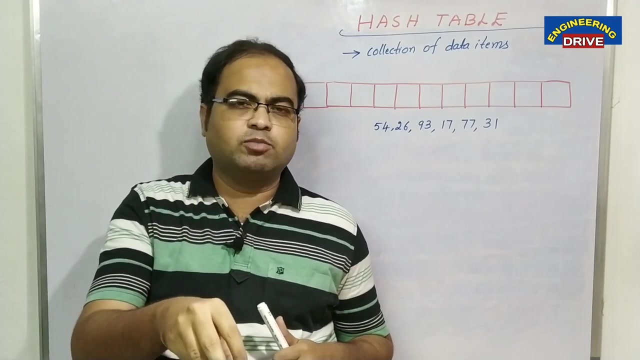 My dear students, first of all, what is a hash table? A hash table is nothing, but it is a collection of data items. What is a hash table? It is a collection of data items, or simply items. Ok, The main purpose of storing the items in a hash table is to find them later very easily. 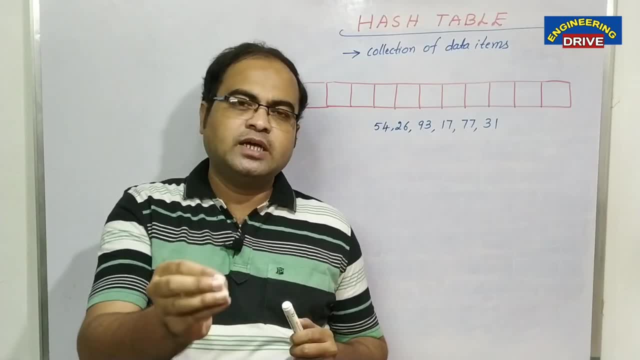 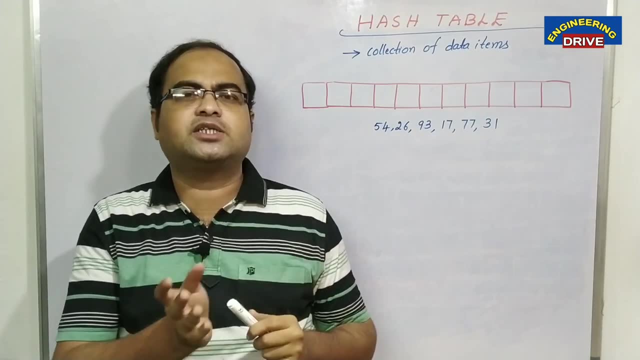 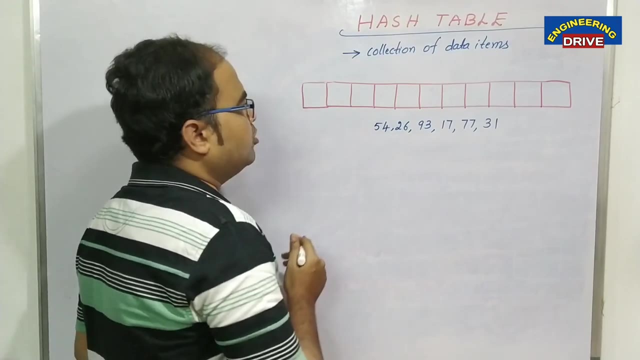 That is the main purpose that we will use hash table to store the items. Ok, now let us take one hash table now. I will show you first of all how the hash table will look like. Hash table will look like similar to that of an array. in our programming or in our data structures, we have arrays. 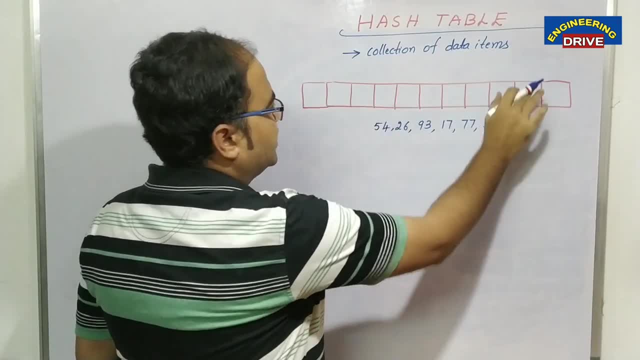 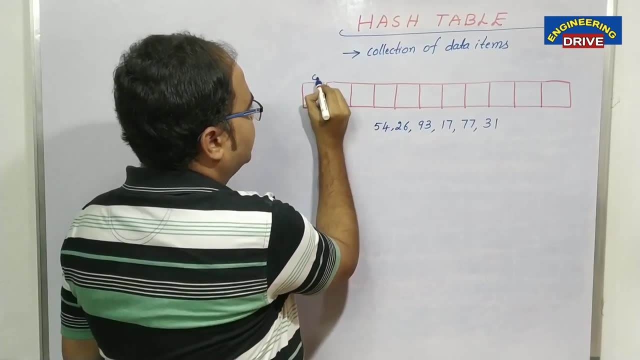 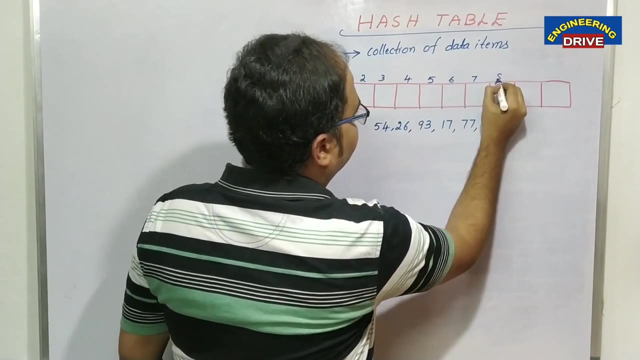 Similarly, our hash table structure. also This is a hash table and this hash table is nothing, but it is a combination of slots. So this is slot number 0, 1, 2,, 3,, 4,, 5,, 6,, 7,, 8,, 9, 10.. 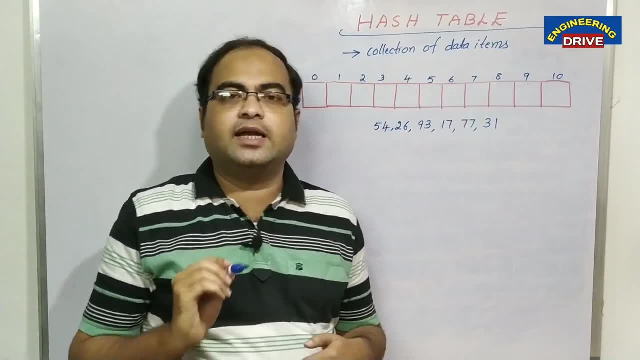 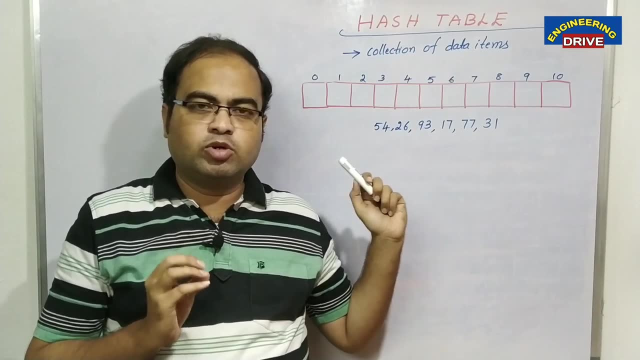 Now we can see this is a hash table of size 11.. So what is the size of this hash table? 11. Which means we can store 11 items in this hash table. Ok, and why we have named this: slots as 0,, 1, 2.. Because it is the rule of a hash table Slot number. first slot will start with the index 0.. Second slot start with the index 1.. Third slot will have the index 2, like this. So a hash table is a collection of slots. 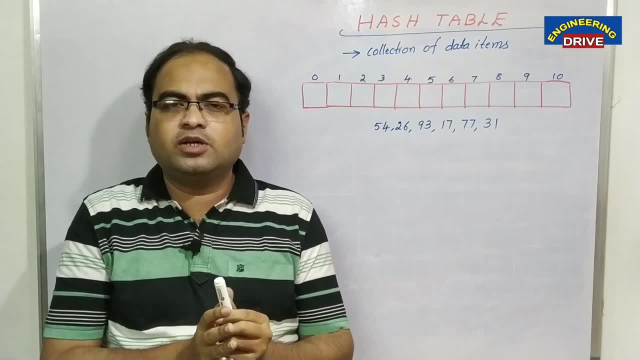 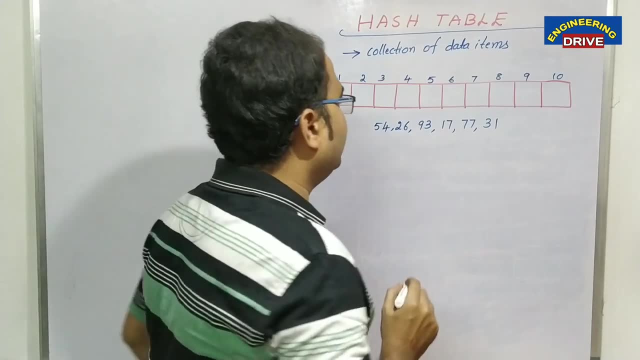 At the starting, the hash table is empty. We can see that there are no elements in our hash table At that time. how to find out whether our hash table is empty or not? If the hash table contains slots. If the hash table contains slots- empty. 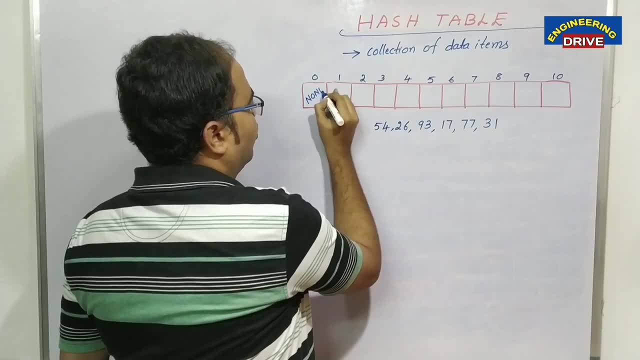 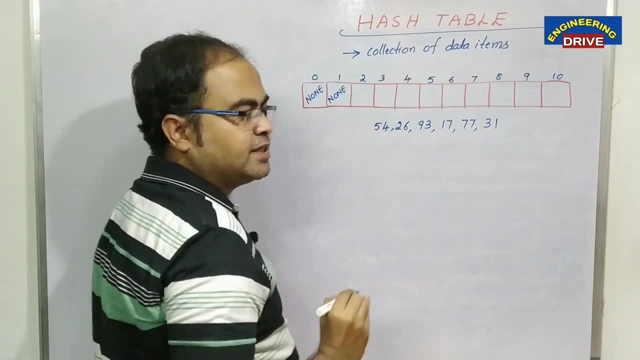 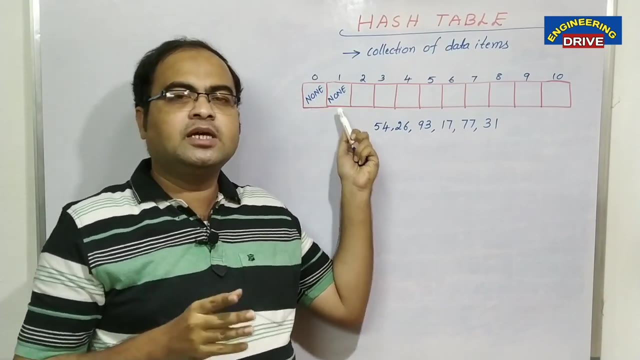 Then it is specified with the word none- N-o-n-e none. Here also we can write none. So what none indicates? None indicates that particular slots in the hash table are empty. Which means now we can see: slot 0 is empty, slot 1 is empty. 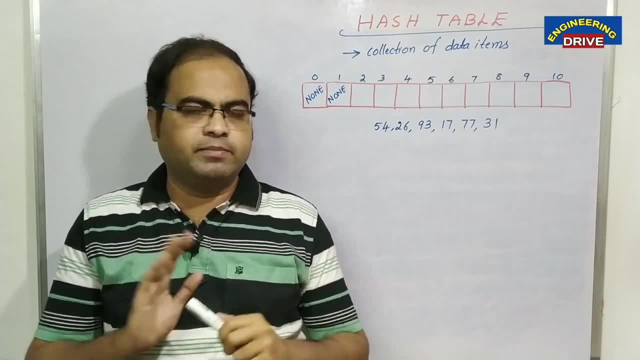 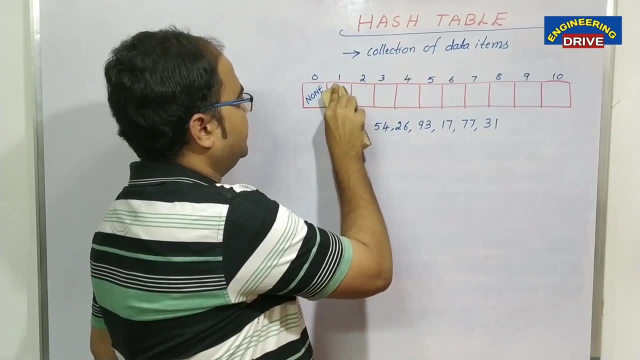 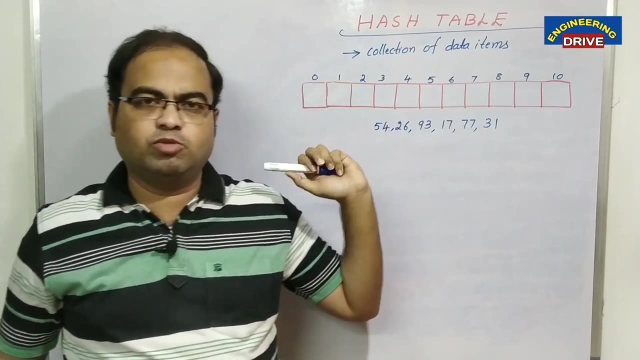 And so on. all the 10 slots, all the 11 slots are empty. Ok, now, next point. This is about hash table structure. My dear students, Now I want to store this set of elements in my hash table now, Because the purpose of hash table is to store the elements or to store the items. 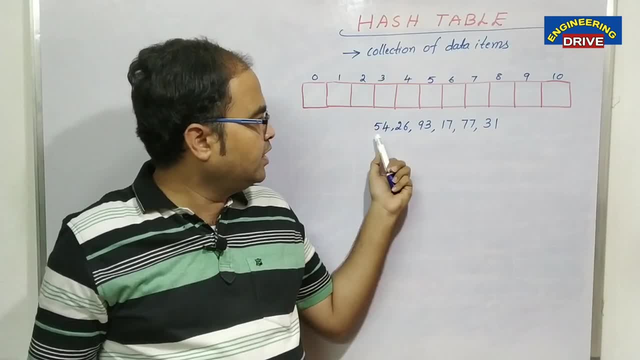 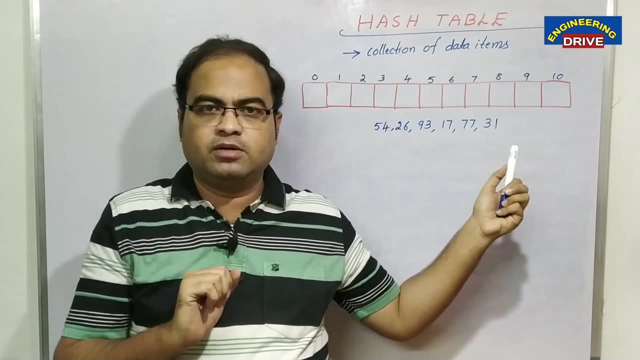 Now I want to store this set of items. How many items are there? Let us take- I have taken 6 items. This 6 items I want to store in my hash table. What is the size of my hash table? 11.. 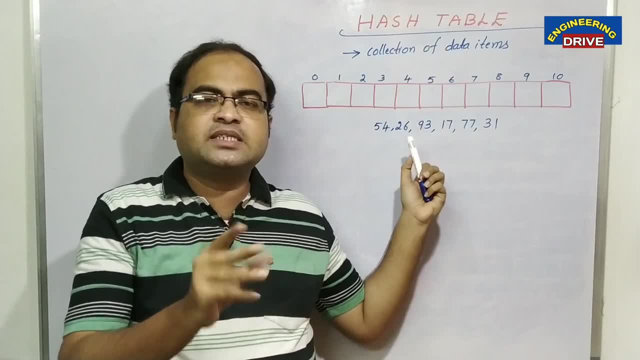 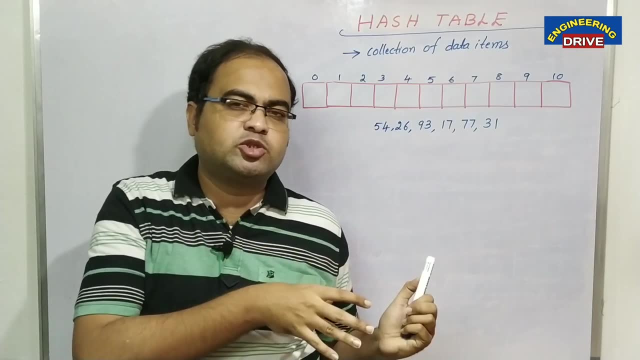 There are 11 slots And how many items? 6 items Now, 11 slots, 6 items. So how many slots will be empty if I store these 6 items, 5 slots will be empty Now. I should decide now. 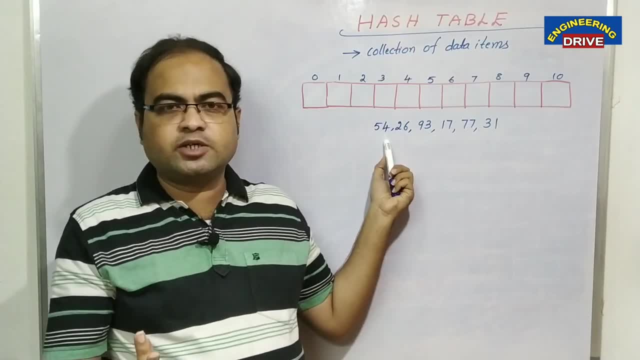 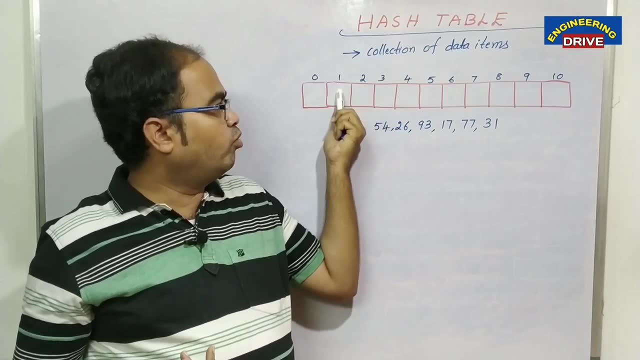 What? Where to store 54?? Casually I cannot store 54. I cannot store in any slot. It is not in my hand. 26 can I store in one slot, number 1?. Can I store 93 in slot number 0?? 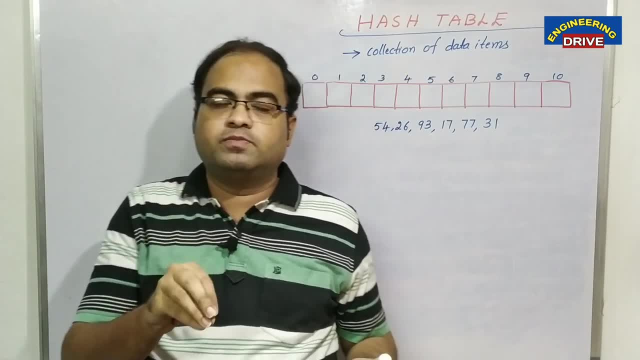 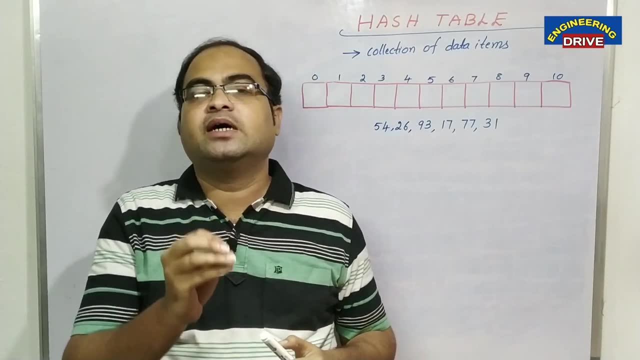 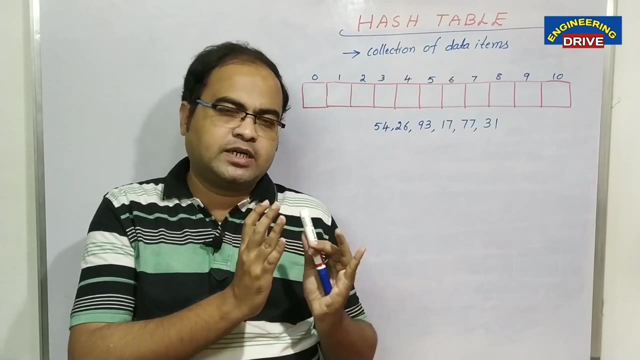 No, How, sir? It is not possible now, sir. Now, The process of deciding where to store the items in the slots is known as hash function. What is hash function, you know? Or what is known as hashing technique. Now we got idea, we got clarity about hash table. now 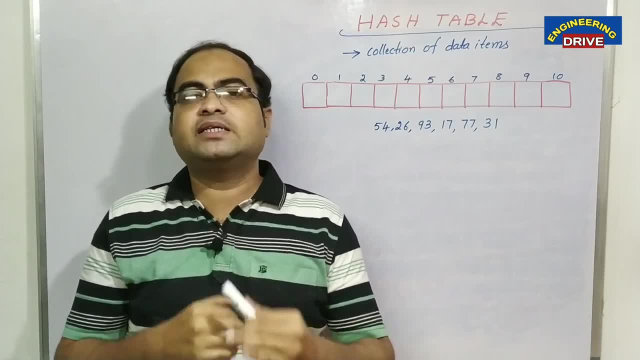 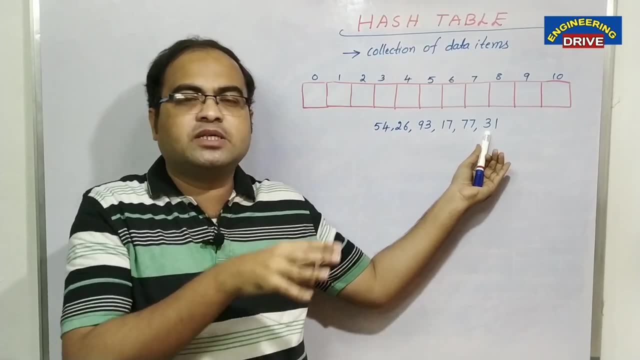 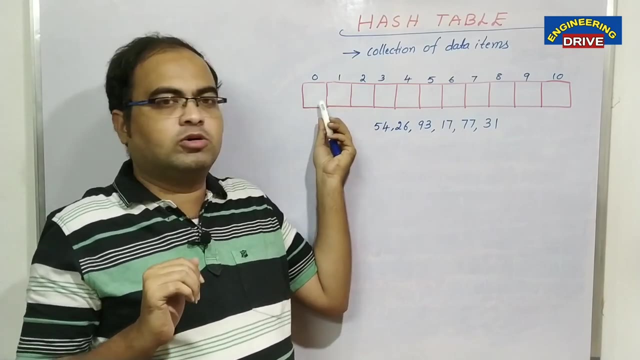 We are moving to second step now. What is hashing Or what is a hash function? Hashing is the technique which is used to decide where to place this items in the hash table. Suppose if I got the confirmation that 54 should be placed in slot number 0.. 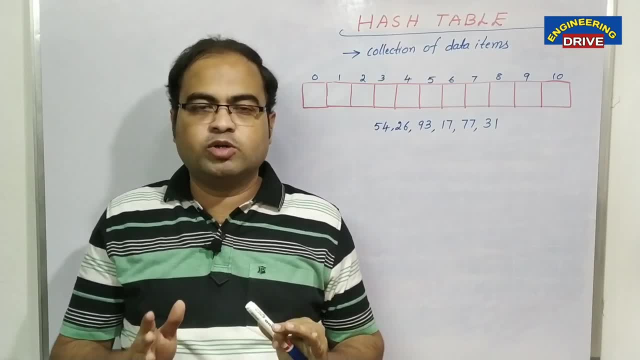 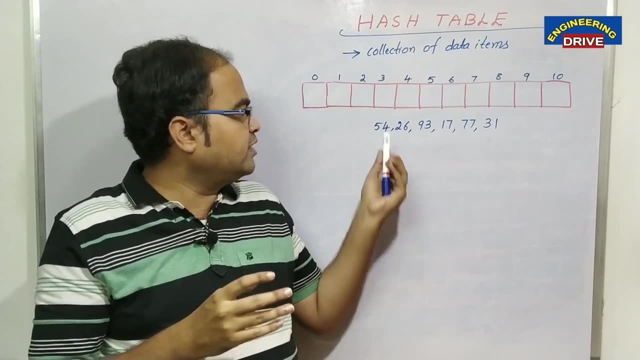 Then what I am doing? I am performing hashing. Ok, Now to perform hashing, I should use some function. I should use some function To find out that 54 should be placed in which slot, 26 should be placed in which slot. 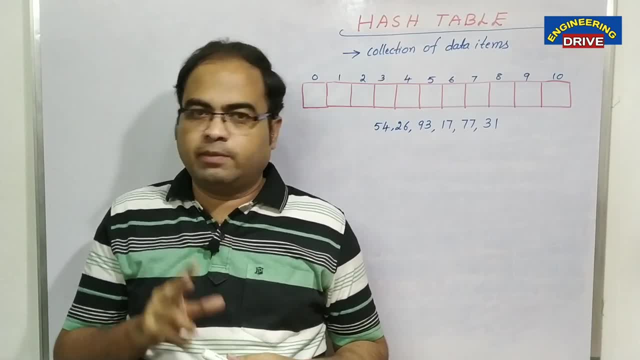 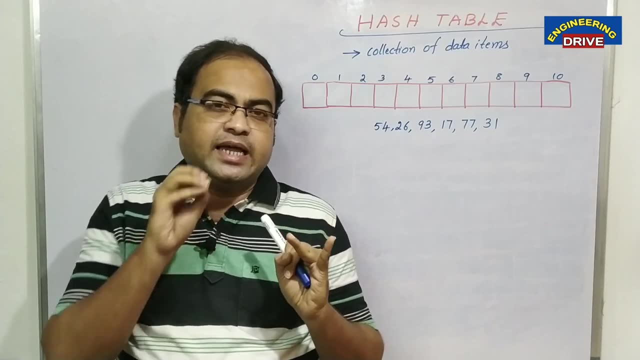 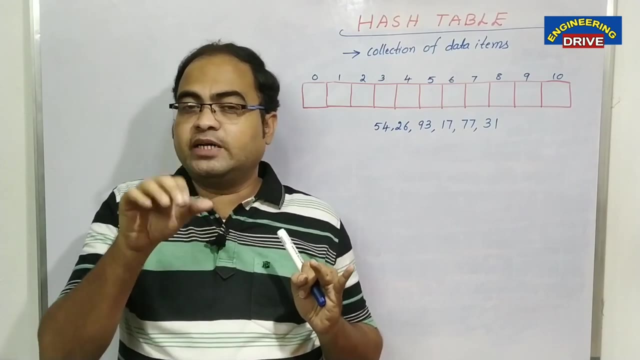 We call this function as hash function. My dear students, You got clarity about hash table, First point. Second point: Where to position, Where to position the elements in the hash table, Where to position the items. This technique is hashing. Now to find out to implement the concept of hashing. 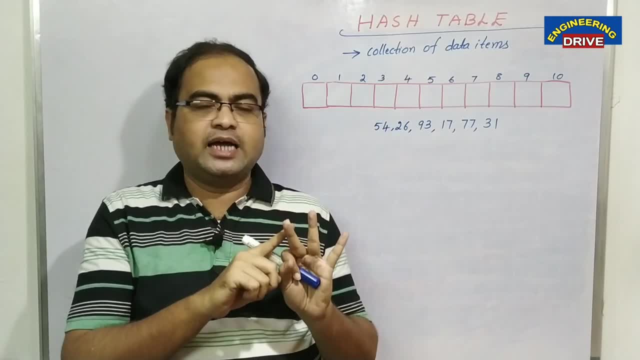 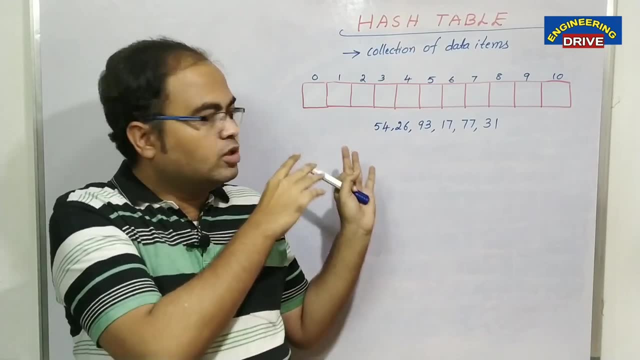 We need to use one function. We call this function as hash function. These are the three things: Hash table, Next Hashing, Hash function. Ok, Now. Now we will see one example. now. With this example, it will be cleared that. 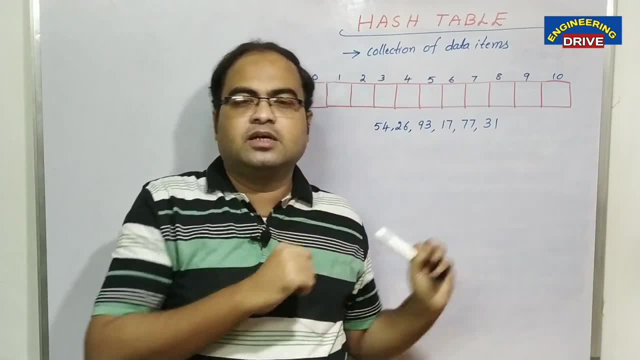 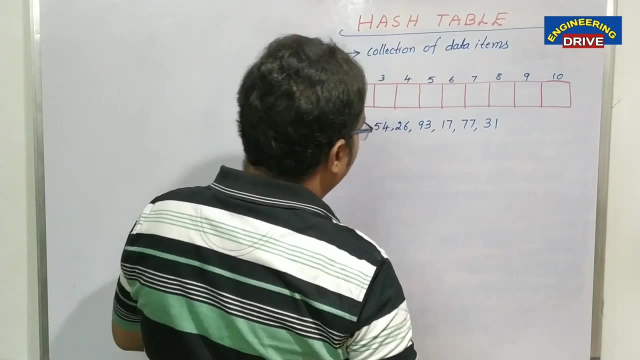 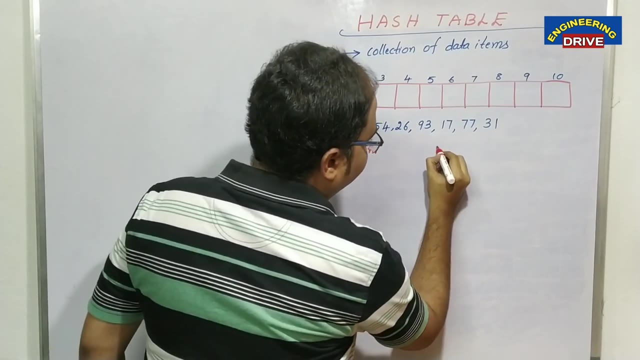 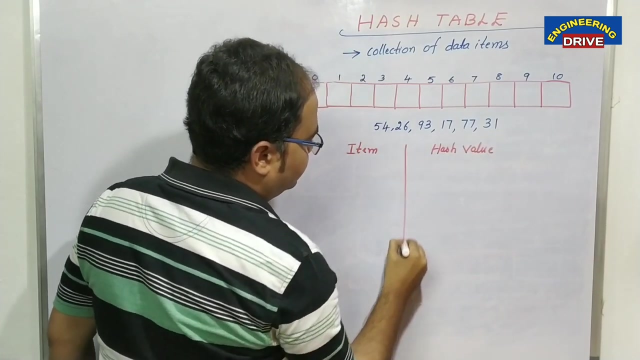 How to position this 6 items in this 6 slots of our hash table. Ok, Now, my dear students, Let us take. these are our items: Item Left side And here Hash value. So First I want to 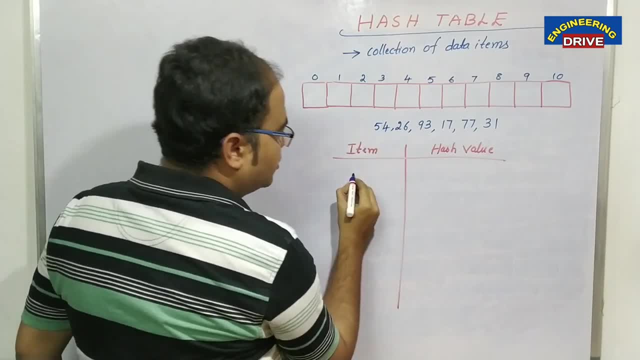 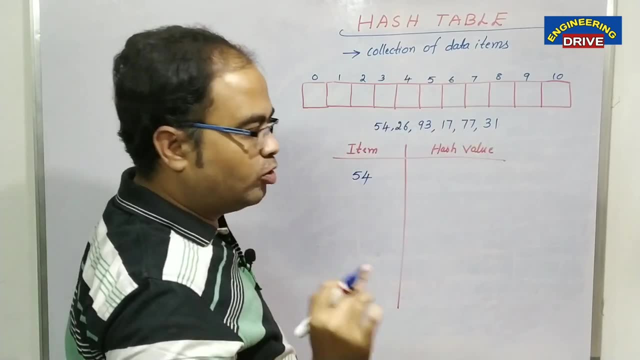 Know Where to position this 54 item. So I am writing here 54.. So This 54 item should be placed in which slot? That is my question now. Ok, Now You people will get doubt, Sir. 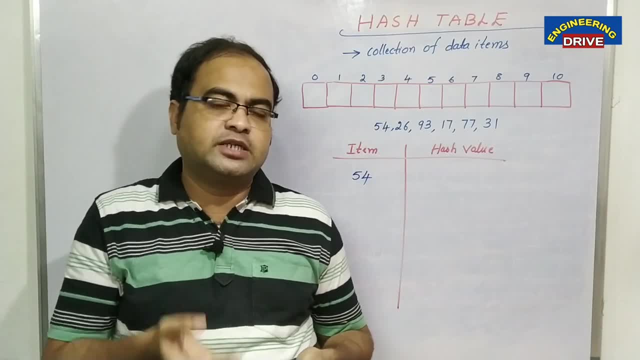 How to place this 54 in this slot. You told that we should use hashing. now We should use some function. Can you give an example? Now, All of you see this example. This 54 is there now. Now I will get doubt. 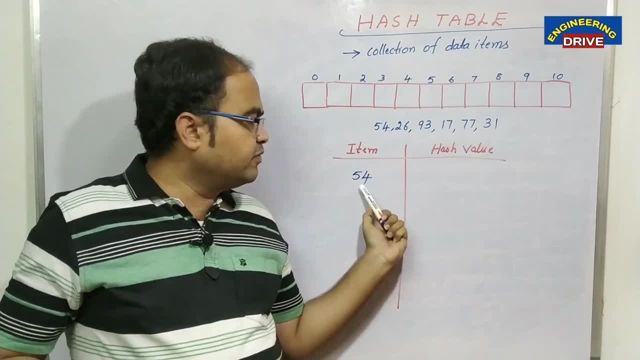 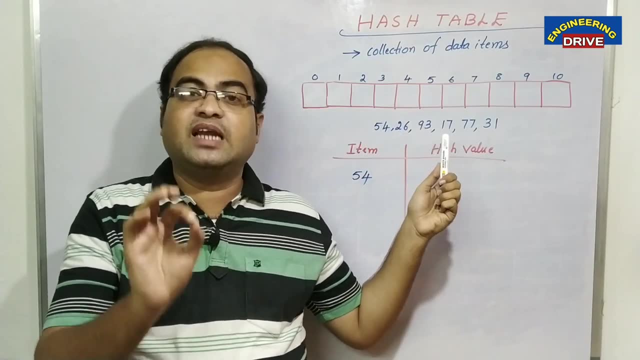 Where to place this 54. In which slot? Now, First number 54. I have selected, First item 54. I have selected. Ok, What is the size of this hash table? The size of the hash table is 11.. Don't say 10, my dear students. 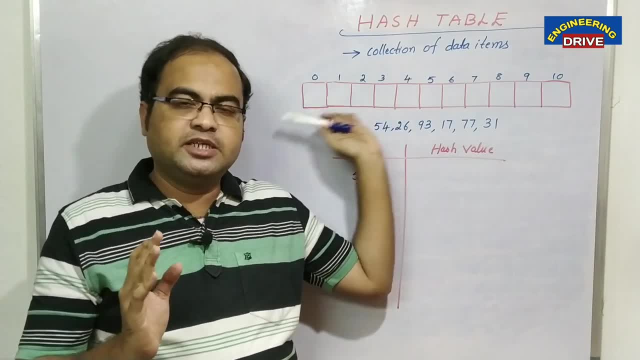 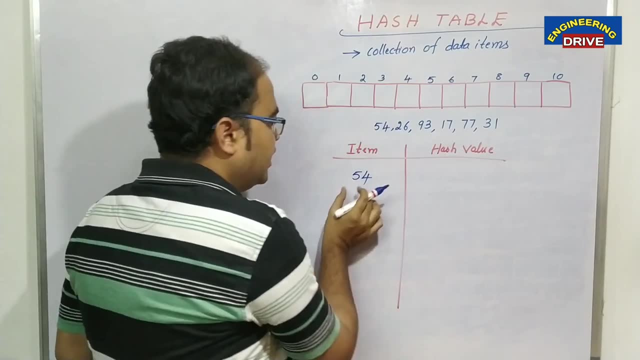 Because 10 is nothing but the slot number. 0 to 10 means how many slots? 11 slots, So The size of our hash table is 11.. So Take this number 54. Divide this number with 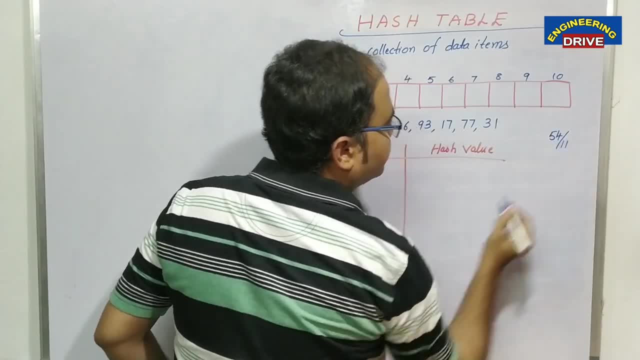 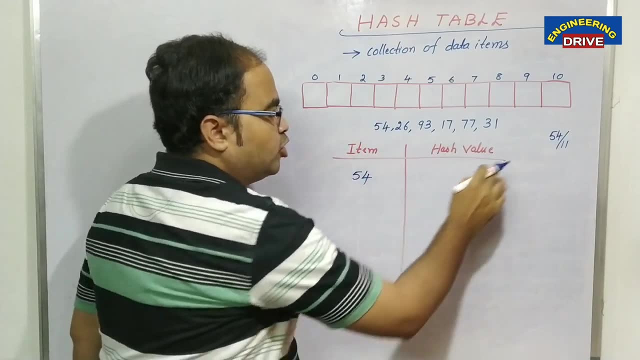 The size of the hash table, That is, 11.. Now, Once you divide, You should take Not quotient as the answer. You should take Reminder as the answer. Now, When you divide 54 by 11.. Ok, You know. 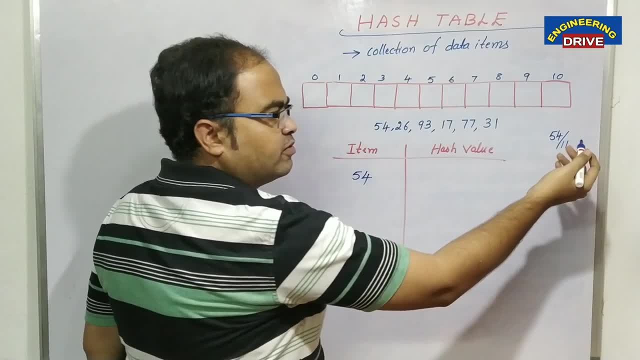 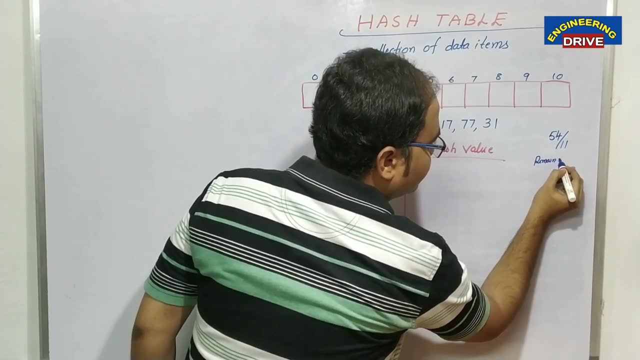 You will get quotient as Something. 4 point: something. You will get quotient, But What you will get reminder? You will get reminder As 11444.. Which means You will get reminder 10.. Ok So. 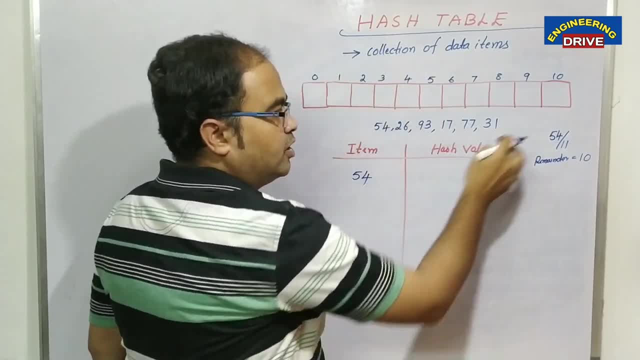 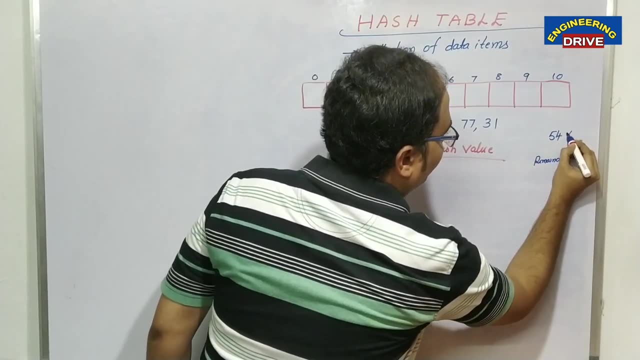 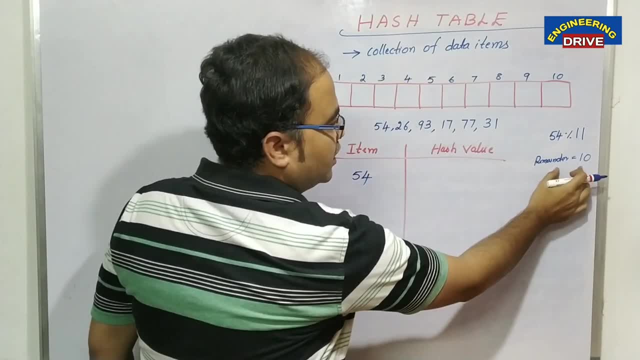 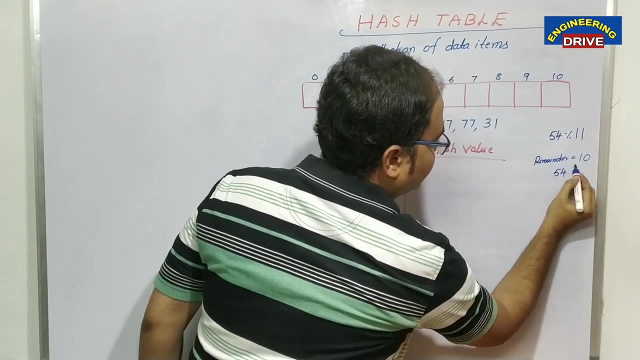 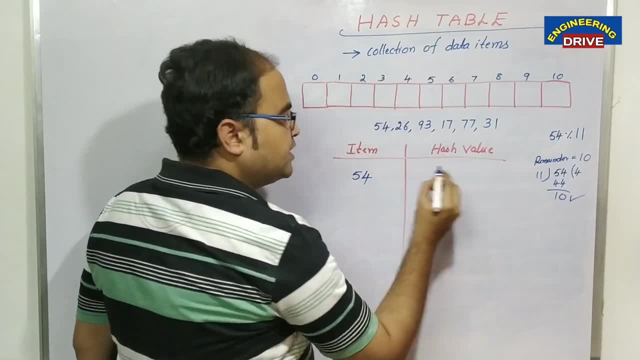 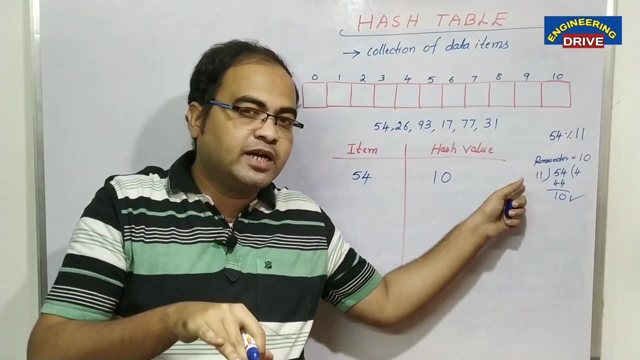 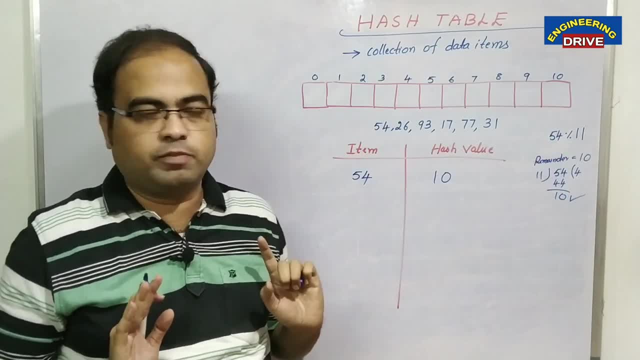 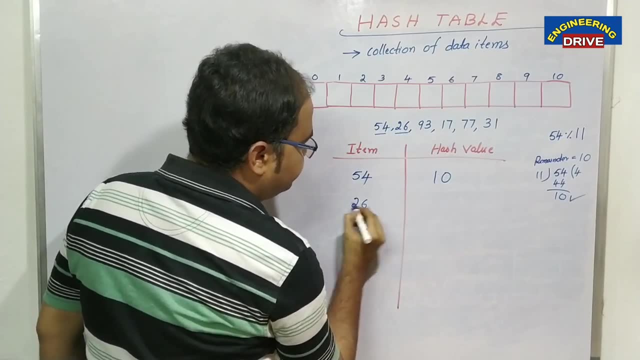 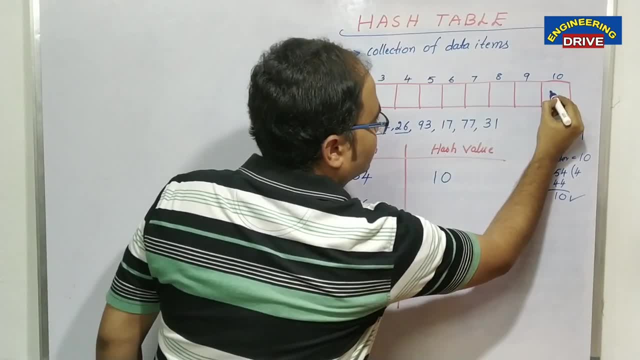 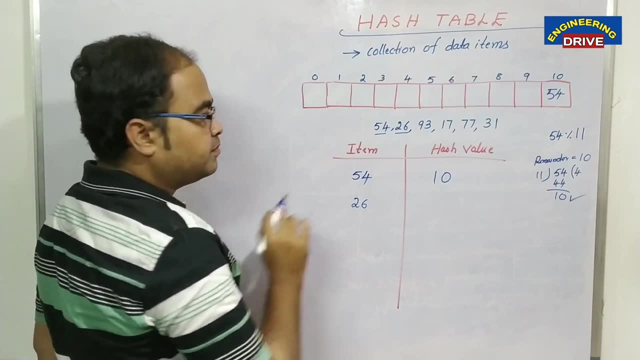 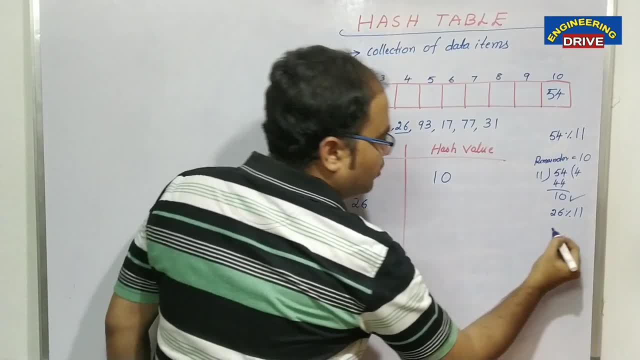 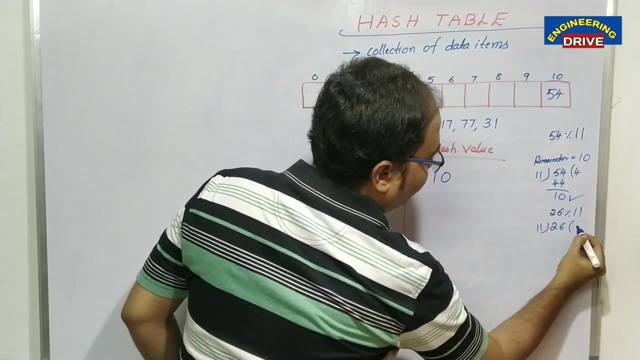 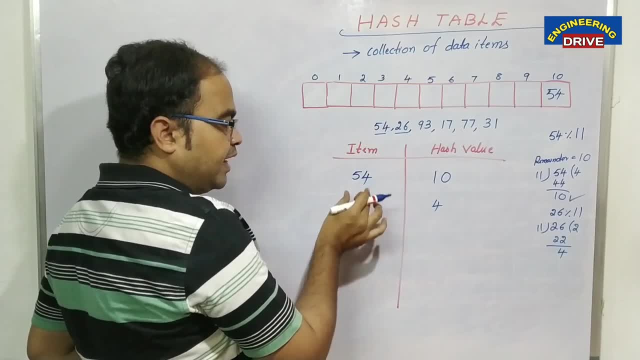 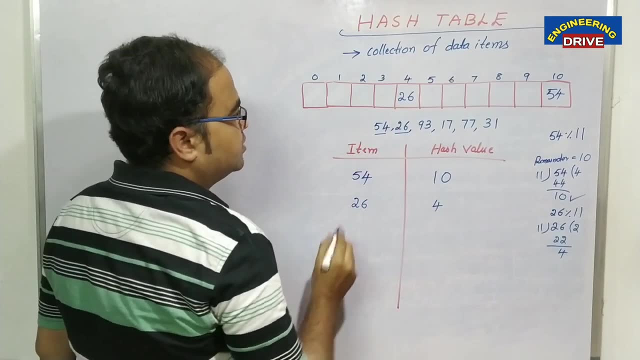 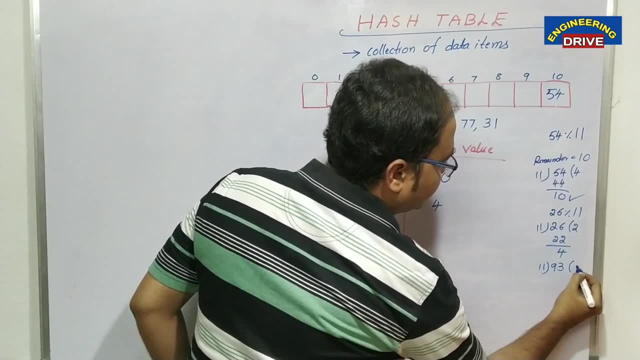 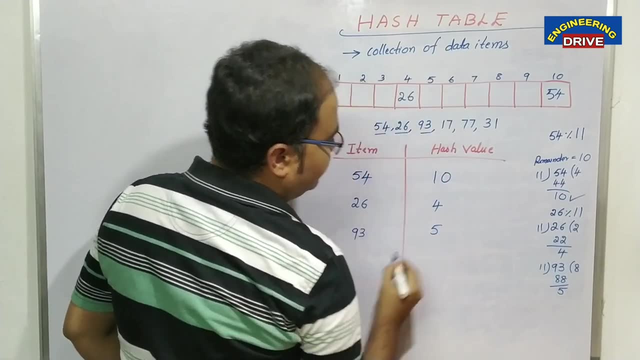 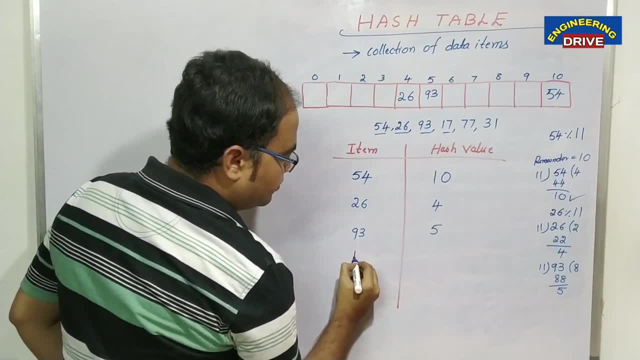 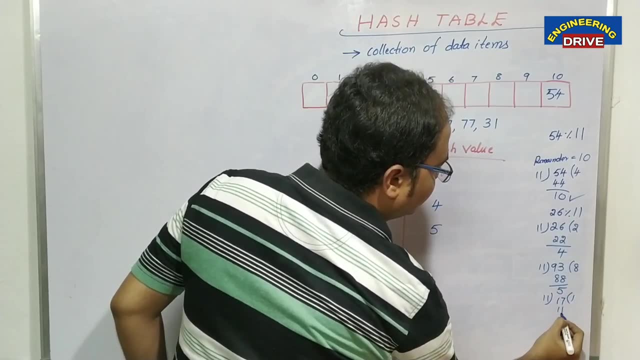 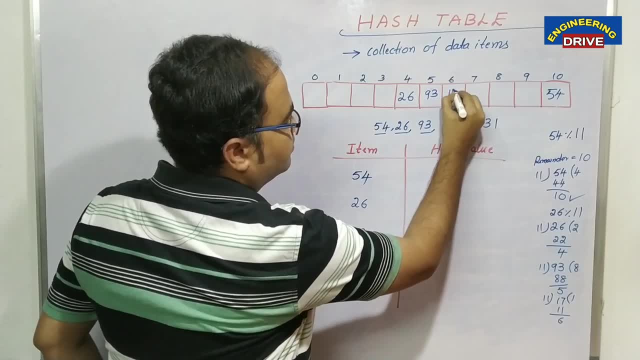 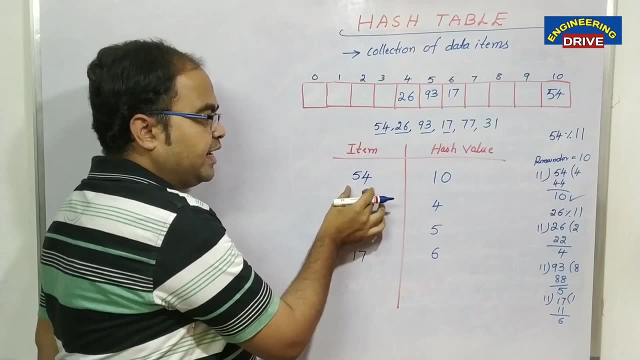 1. 1. 1. 1.. Hopefully the concept has been clear to you, So I am not doing any extraordinary work here, simply what I am taking, taking the item, dividing it with the hash table size and getting the hash value as the reminder. 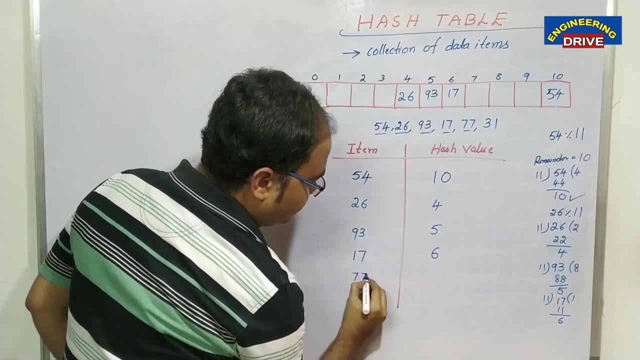 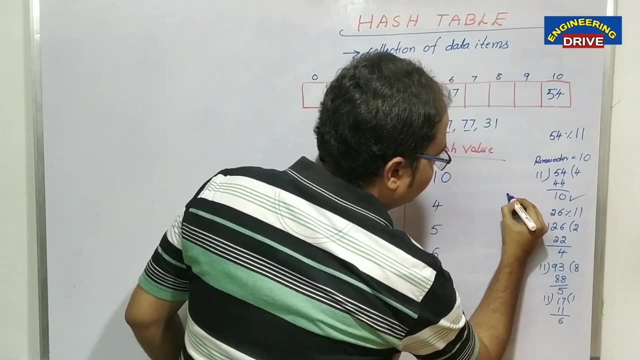 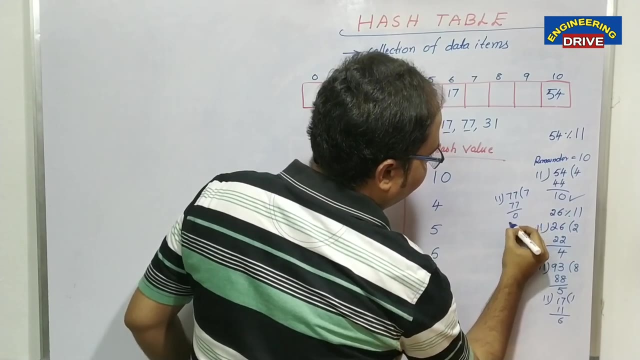 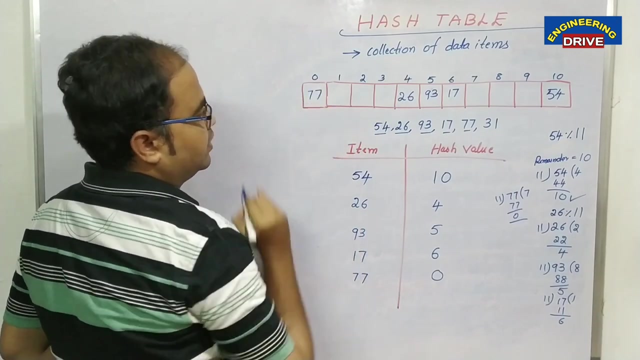 Next, fifth item: 77, 77 divided by 11, again what we will get to. so 77, 11, 11, 7, 77, which means the reminder will get 0.. So the hash value we got here is 0, which means that the slot 0, you need to store 77, ok, and 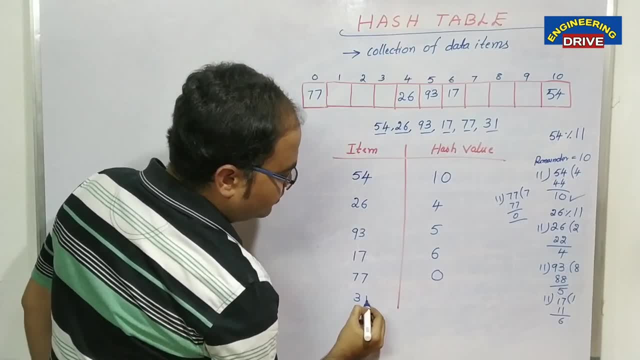 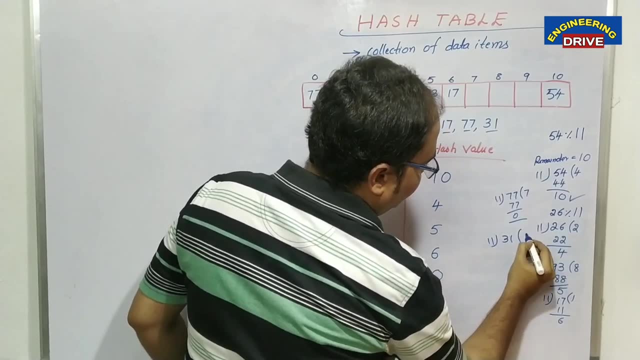 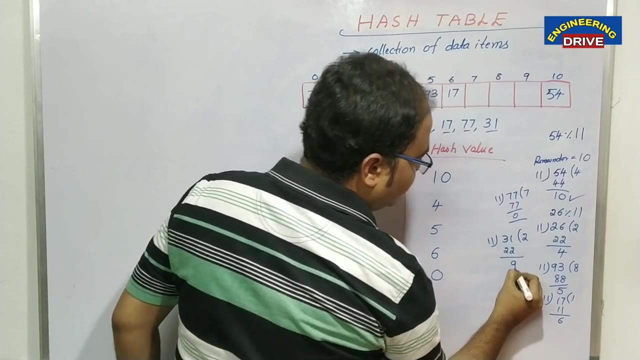 take the last item date, item 31. ok, for the item 31, let me divide it: 11,, 11 to 22.. So what is the reminder will get? the reminder will get is 9, ok, So this is hash value 9.. 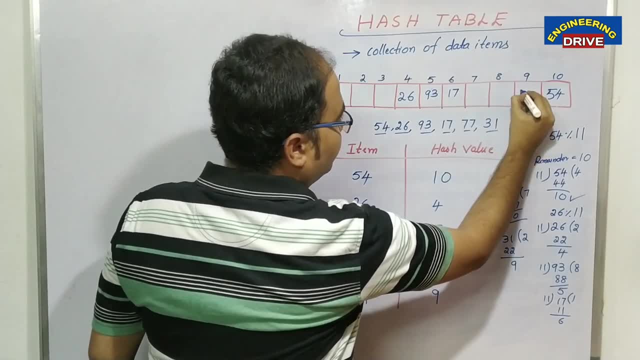 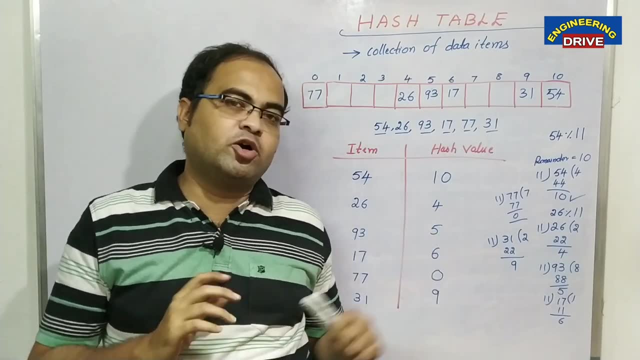 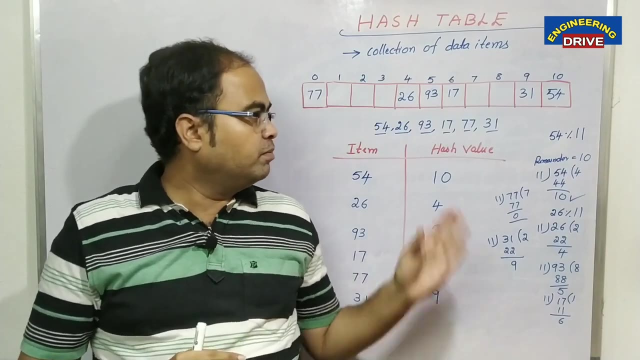 So, which means, at the slot number 9, store the value 31.. So now, my dear students, now you tell me whether the job is easy or not. You people will think I told already at the start of the video. you people might have thought that it will be very difficult topic. 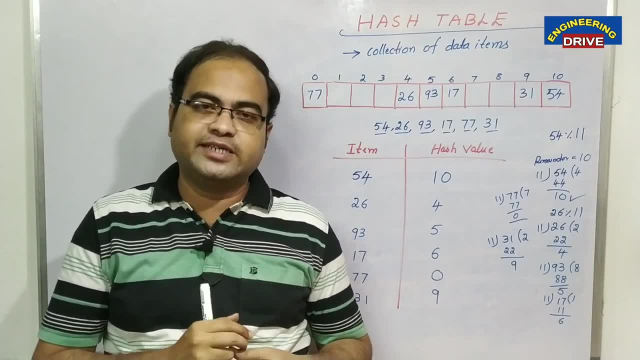 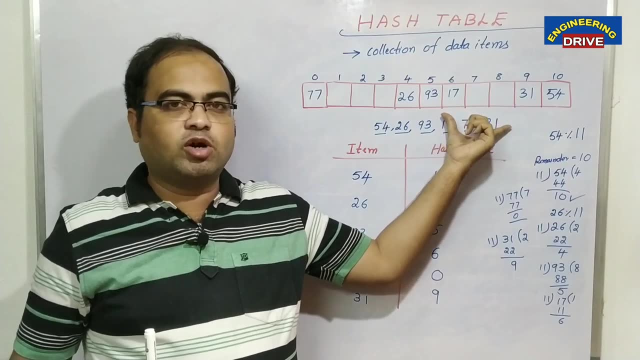 But hash table topic is one of the easiest as well as interesting topic in data structures. So in this way we need to store our values. So 6 items placed in 6 slots. ok, How? How many slots are selected, depending on the technique: hashing- 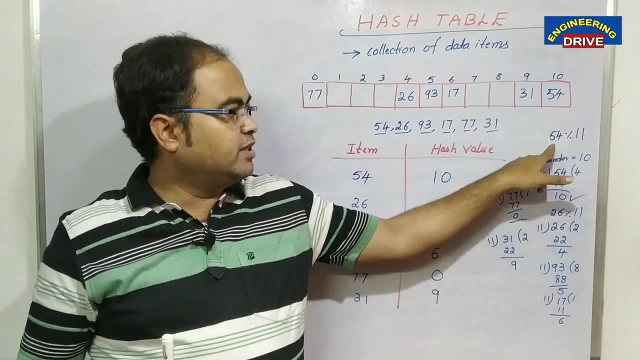 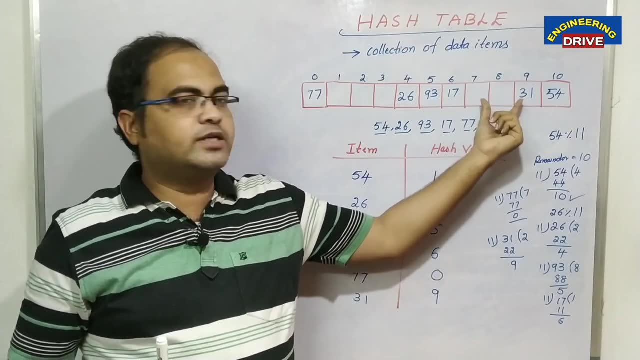 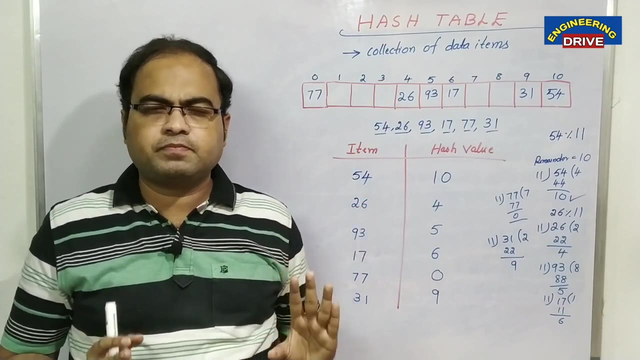 Hashing makes use of a function, hash function, that is the mod operator. So here we will take the item mod table size, hash table size and whatever the reminder we will get, that is our slot number, that is our hash value. on that particular hash value we will keep our data item. ok, clear. 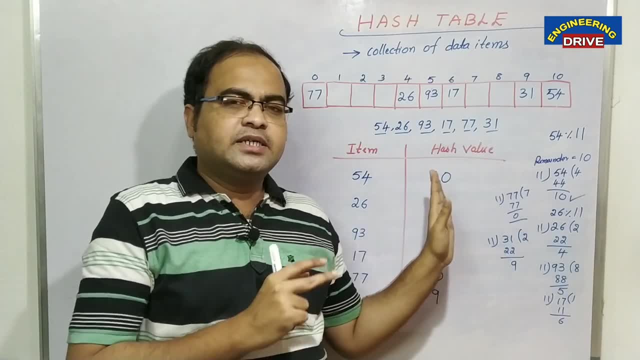 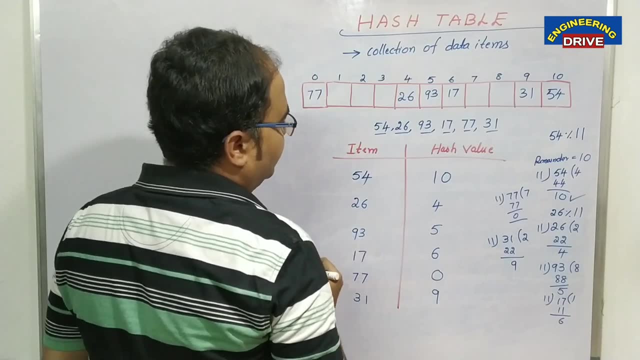 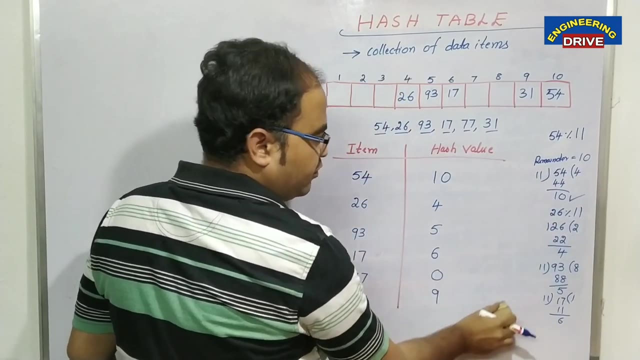 Now, once the hashing is completed, once we have stored the elements in our hash table, We need to find out one more one thing at the end. What is that one thing means? let me erase this one. let me- hopefully you can pass the video and note down the rough work also, if you want- ok. 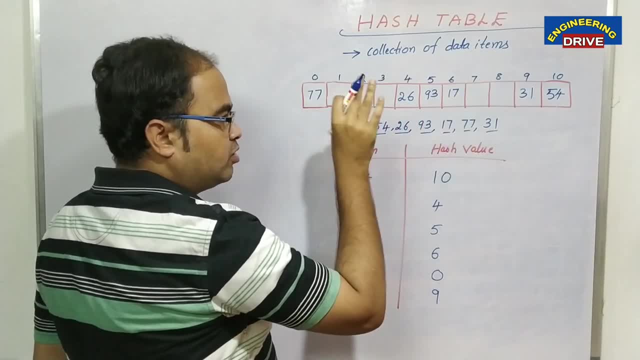 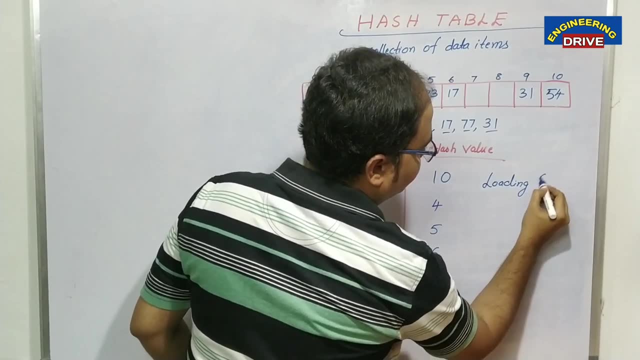 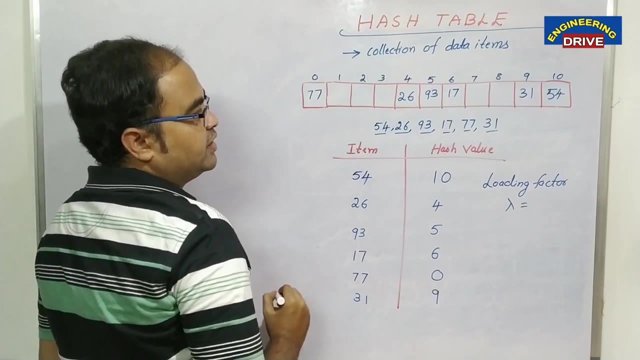 Once we have completed, once we have filled the, once we have stored the items in the hash table, we need to find out one thing, that is, loading factor. Yes, Yes, Yes, Yes, Yes, Yes. Loading factor is indicated with the symbol Lambda. 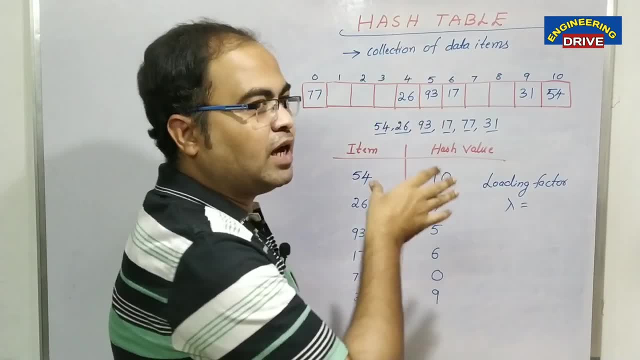 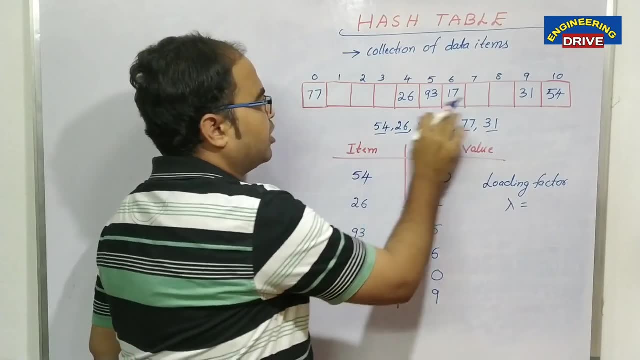 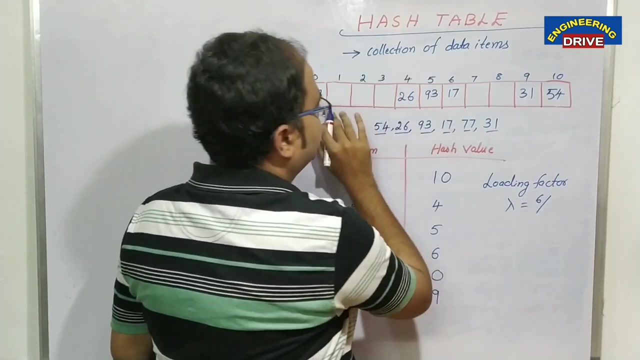 What is loading factor? you know, loading factor means how many items are present in the hash table divided by the hash table size, which means you can see the total number of items available in our hash table: 1234566 divided by the hash table size. that is not one. 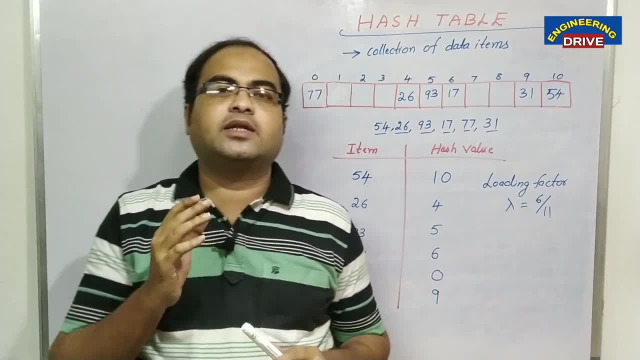 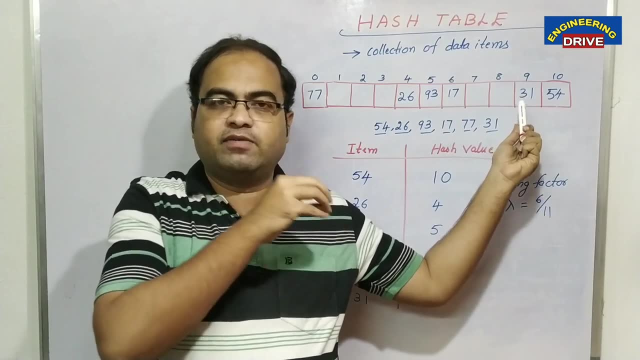 This is our loading factor. Loading factor indicates the load in our hash table, When we can say how much load is there in our hash table depending on the items that are available in the hash table. There are 6 items in our hash table and the size of the hash table is 11.. 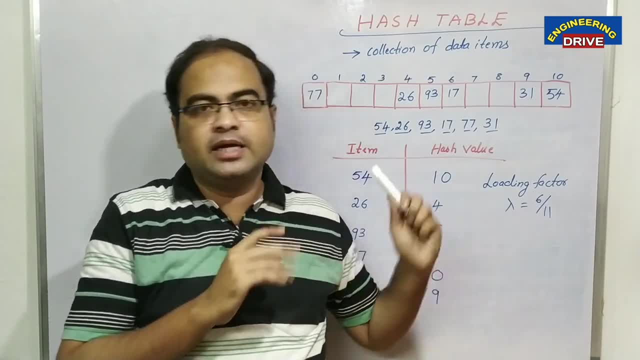 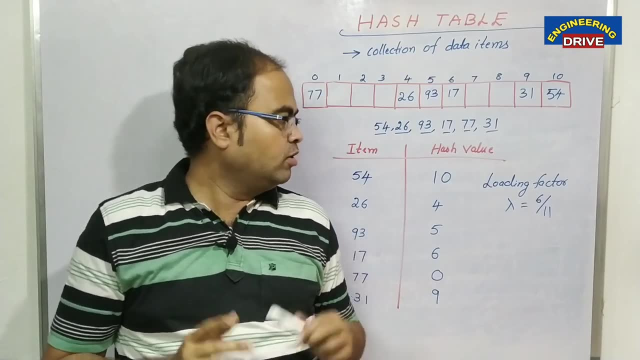 6 divided by 11 is the loading factor which is indicated by lambda. ok, And one more last point I want to discuss- then I will close this. today's video, My dear students, is. some students can ask you one more question: what is that? 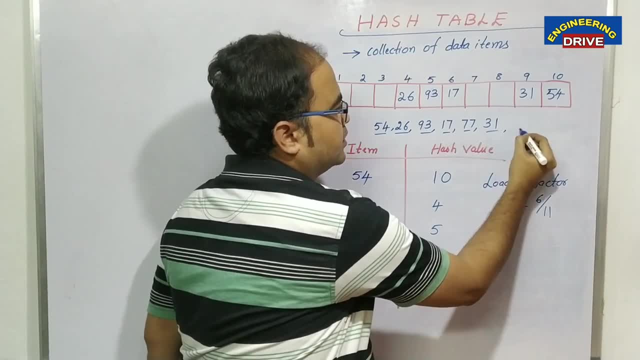 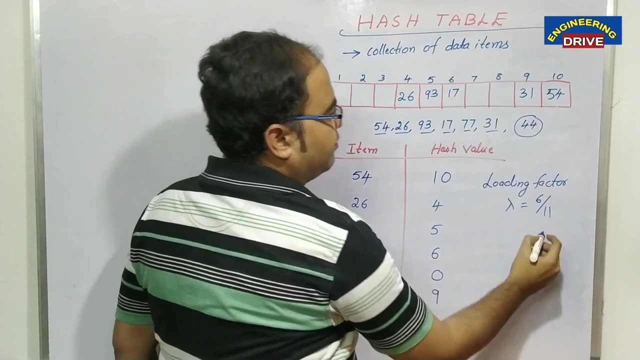 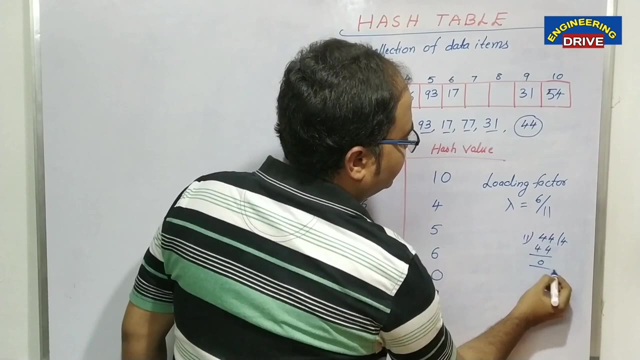 Sir, let us say one more element is there here. Let us say 44 is available. one more value: 44. Now 44 item is there, if we divide 44 by 11. So at that time also we will get reminder 0, which means 44 should also be placed in. 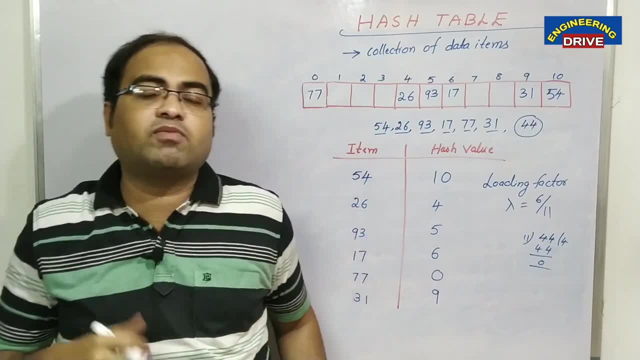 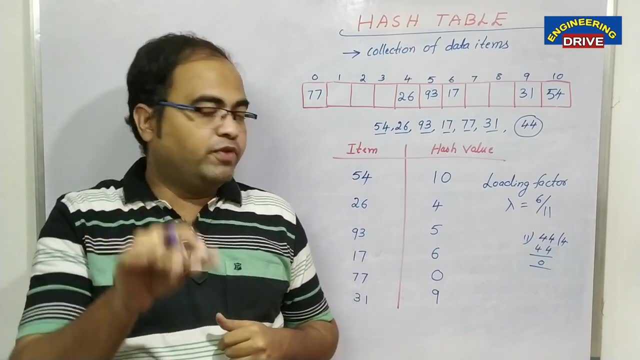 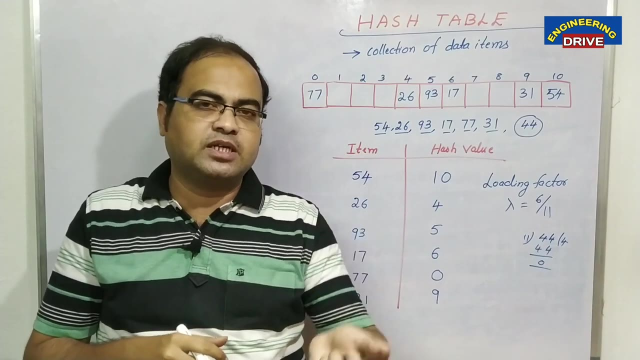 the slot number 0. But already element item is there in the slot. no sir, what to do at that time? Yes, my dear students, this thing is normal in the hash table. This is one of the problems in hash table When, When we get the second item in the same slot, when we need to place the second item in the 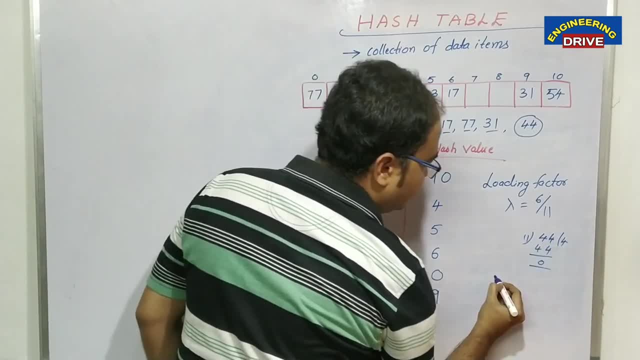 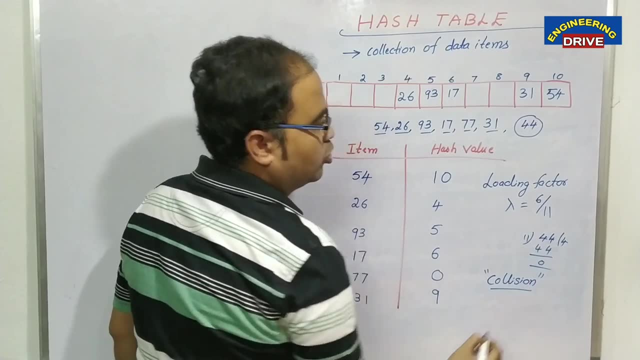 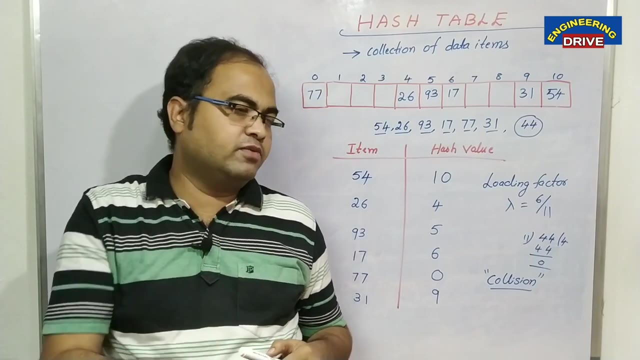 same slot. we call this particular process as collusion. What we call this one Collusion: When already there is item in the slot, when the next item also tries to appear in the same slot, when the next item will appear in the same slot, when you will get the same hash. 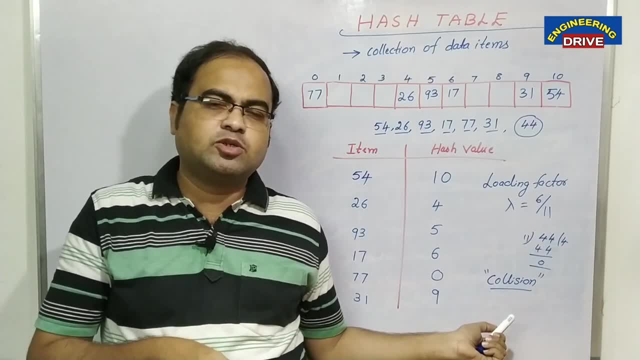 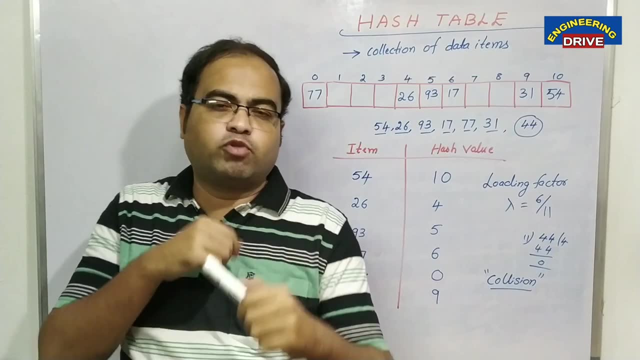 value. We call this process as collision. Why we are calling is as a collusion, because already there is no place for the new element to store in the slot. That is why what will happen at that time when you forcefully want to insert one element in the already present element in the slot, then collusion will happen. 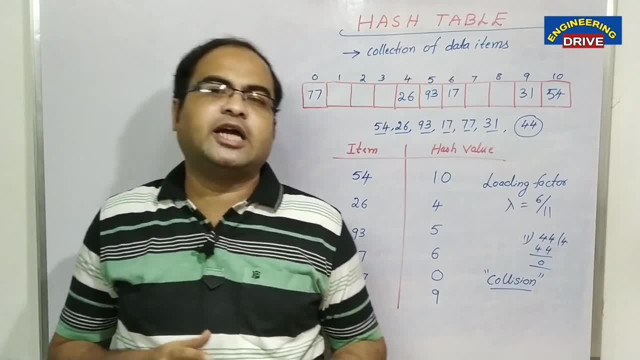 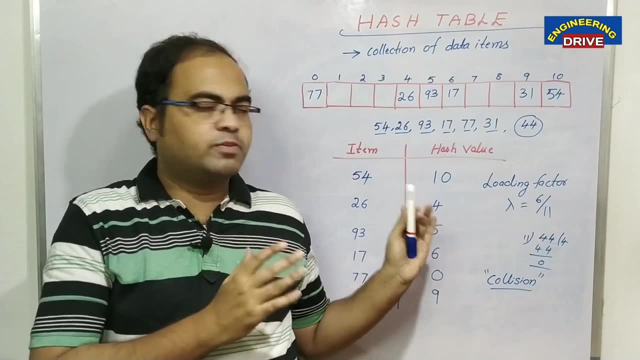 We call this problem as collusion. However, collusion can be avoided by using some other various types of hashing techniques, my dear students. So hopefully the concept of hash table has been clear to you with this example. and again, in hashing also, we can perform starting hashing.